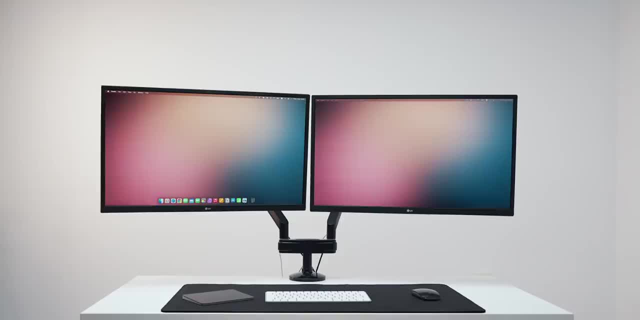 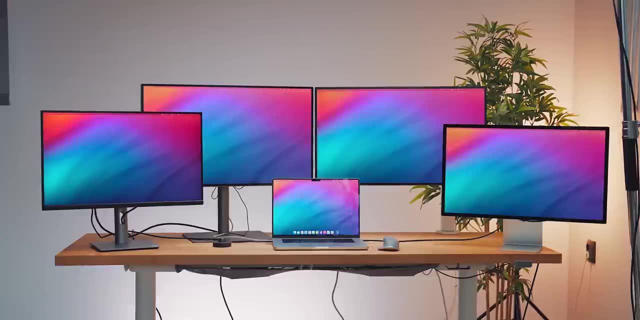 This video is brought to you by Banks. Since the release of my monitor guide video episodes, I have been receiving a lot of questions from viewers about displays for creators. Today, we will take a look at four high-resolution color-accurate monitors, ranging in price from 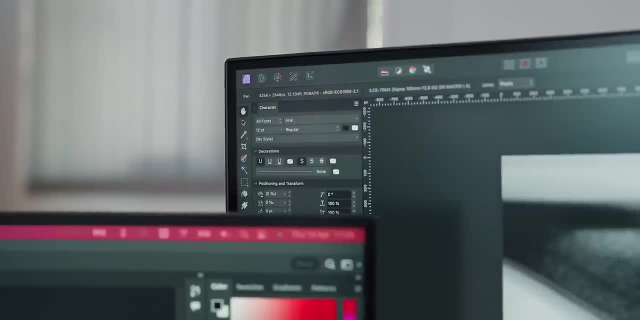 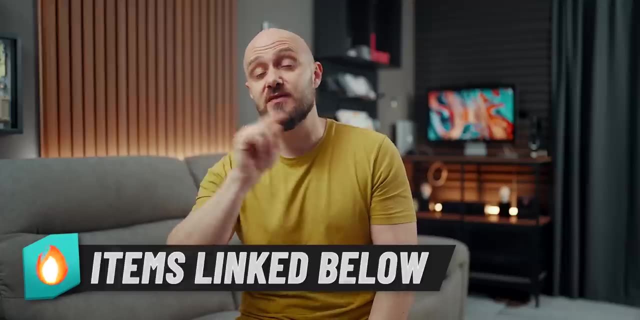 $500 to $1,600.. I will go over the specs, main differences, shortcomings and at the end I'll show you my personal picks from the four. I will also make sure to link all of them, plus some other great monitor choices in the description below. With that out of the way. 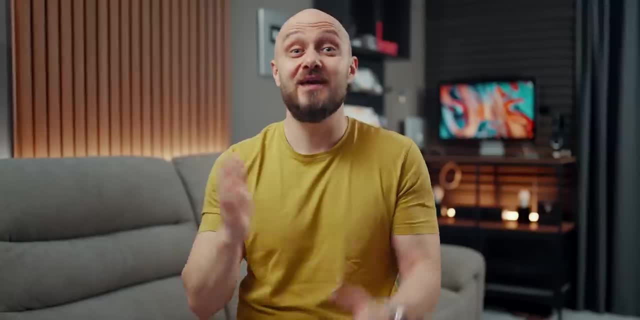 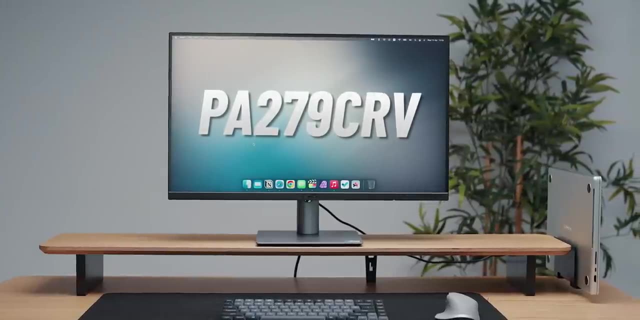 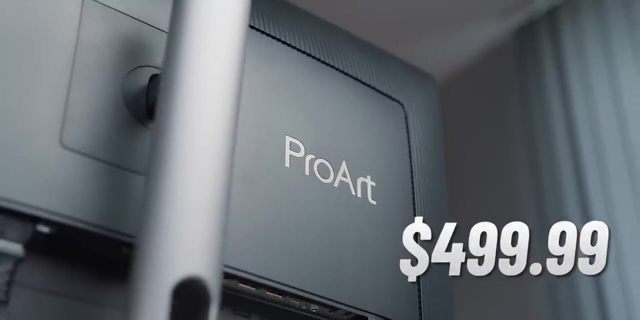 let's check out the four contestants, what makes them special and their respective prices, Starting with the recently updated Asus ProArt Display model number PA279CRV. This is a 27-inch 4K panel that offers a lot for its price, which is $500.. This is by far the cheapest monitor on. 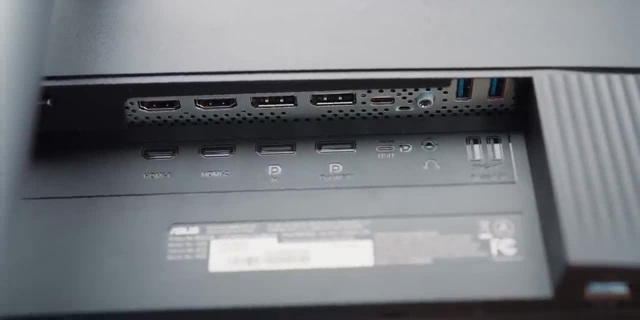 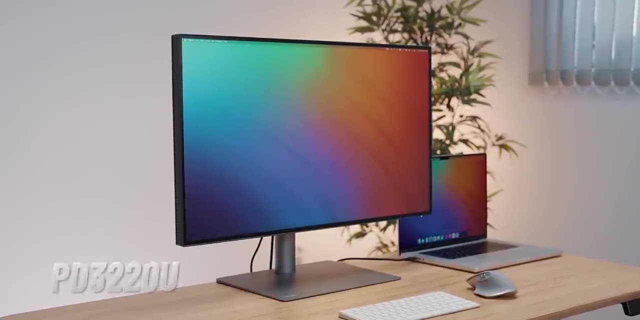 this list, but don't rush into conclusions, as it has a lot to offer. Next up is the old but classic BenQ DesignView PD3220U. This 32-inch 4K monitor has been in the top charts, I believe, since 2019.. We're talking. 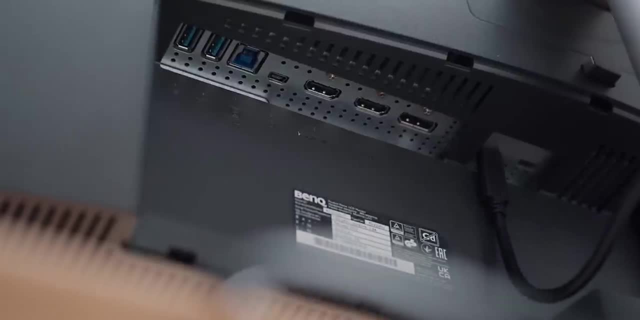 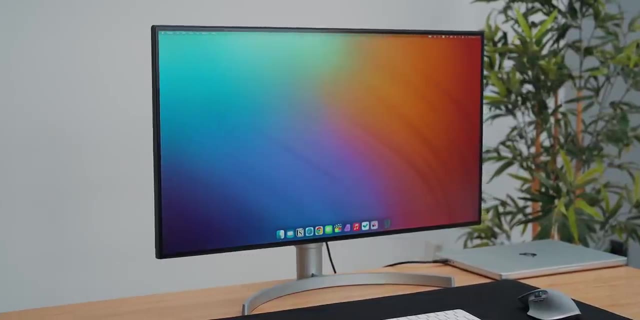 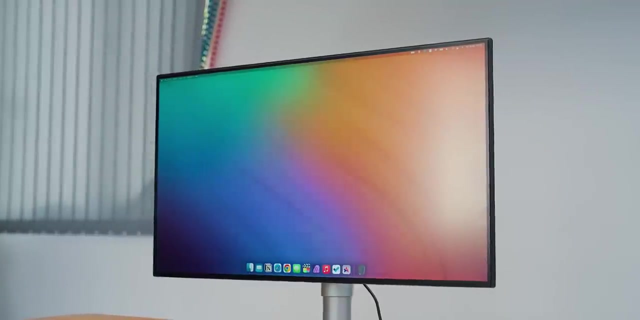 about Thunderbolt 3, daisy chain capabilities, ports galore and more Going up in price. we have another favorite, the LG Ultrafine 32UL950-W, At 32 inches again and 4K resolution. it is yet another golden oldie from the end of 2018 that remains a recommendation of mine. 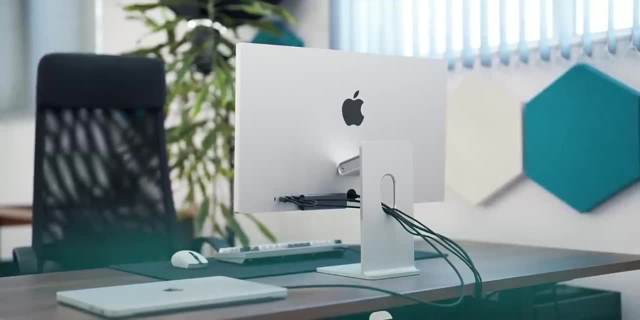 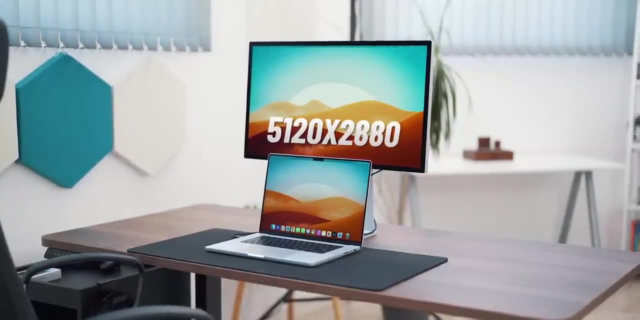 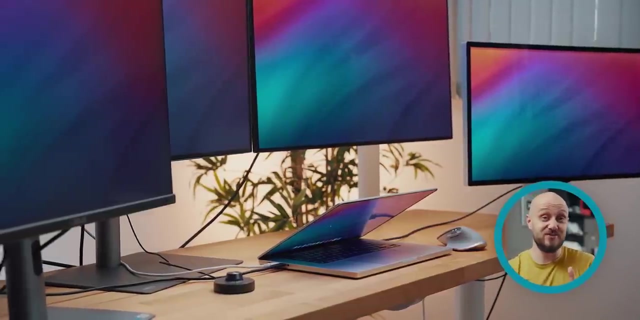 to this day. The final contestant is the controversial Apple Studio Display. Starting with all the extras, this 27-inch display is the only 5K monitor here. I'll leave it at that. Just like in contracts, I shall be referring to all four monitors hereafter as Asus, BenQ, LG. 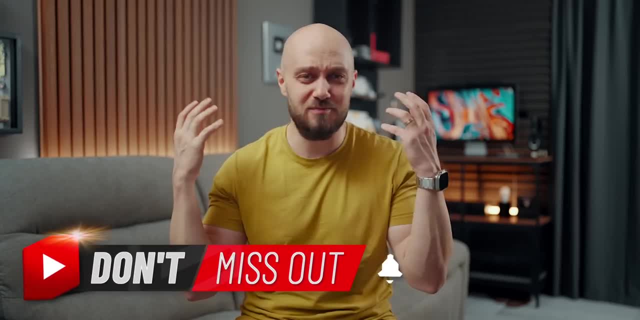 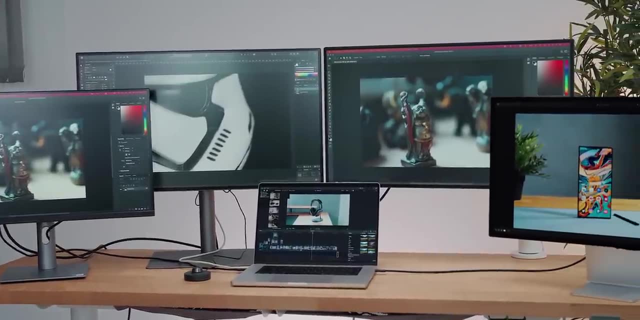 and the Studio Display. By the way, if you end up enjoying this video, subscribe, because why not? So, looking at all four, here are some factors you should consider. All monitors have a 16x9 aspect ratio and all four are IPS running at 60Hz, As they're all marketed as. 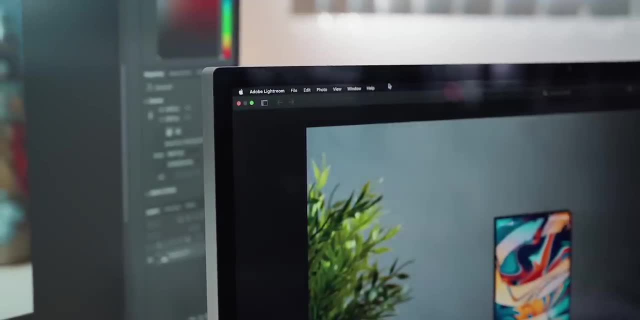 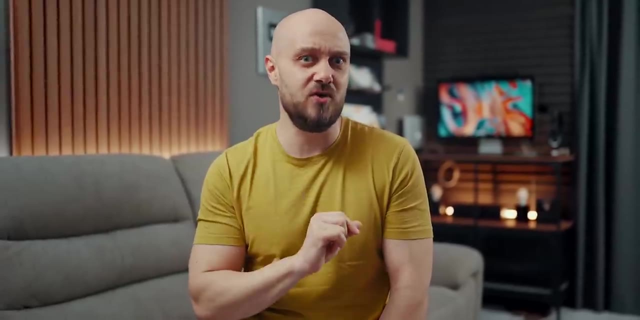 displays for creators. all are factory-calibrated, offering various types of intimidating lingo showcasing how accurate they are out of the box. I trust only one of them, though. The LG and BenQ are both 32 inches, while the Asus and the Studio display are 27 inches. 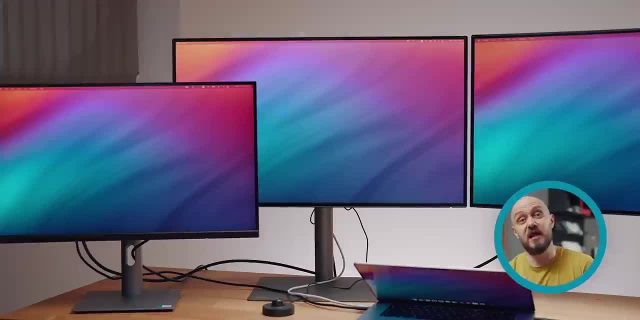 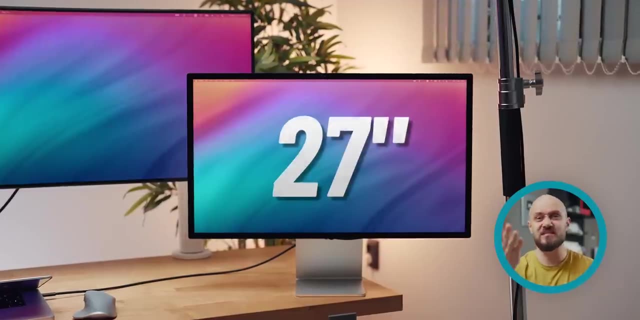 Both of those sizes will serve you well. I have personally been advocating in favor of 32 inches, as it is a tad easier on the eyes when looking from a proper distance, But 27 inches will not be a bad choice either, In fact, if we talk about 4K resolution. 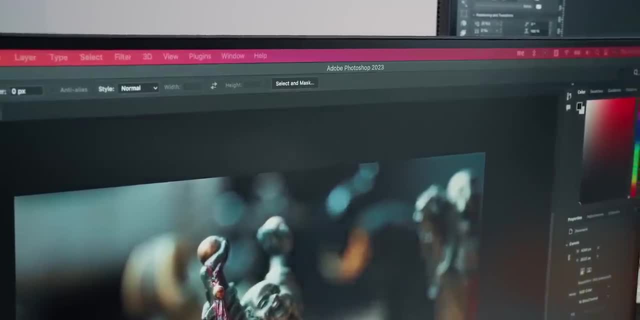 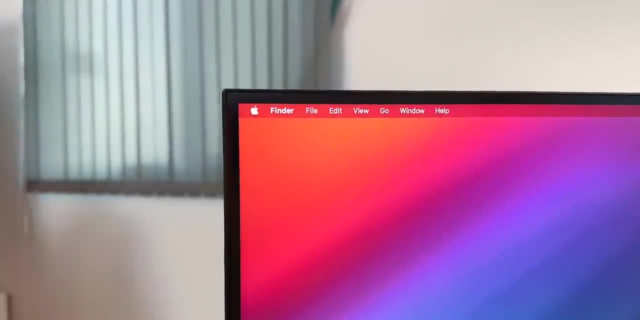 all three, except for the Studio display, will give you a decently sharp picture, where the smaller 27-inch Asus will stand out with a pixel-per-inch density of 163.. The 32-inch choices have 137 PPI, if you're interested, However. 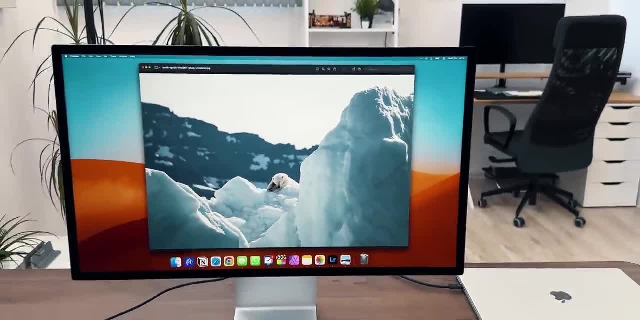 nothing can compete with the Studio display in terms of sharpness, since at 5K you will witness 217 PPI. With the Studio display, you don't have to worry about the sharpness of the Asus and the Studio display, since they are both 27 inches. 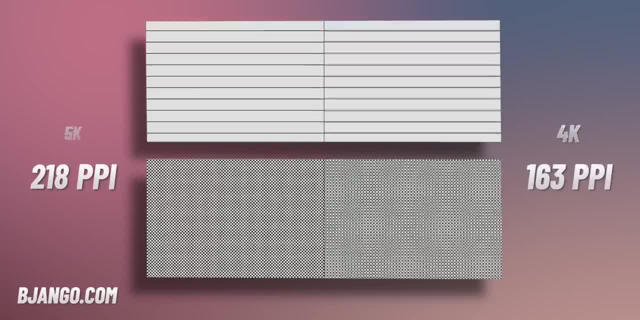 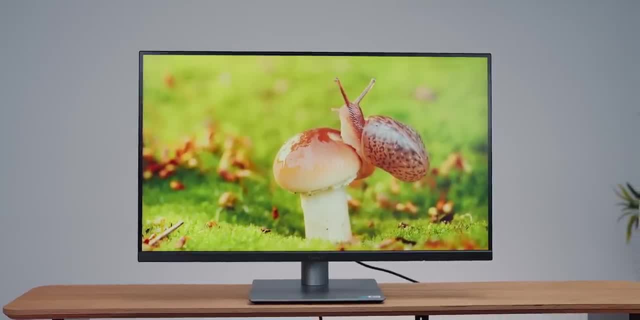 However, nothing can compete with the Studio display in terms of sharpness, since at 5K you will witness 217 PPI. So let's start with the Asus. In terms of panel technology, the monitor covers the most important metrics with flying colors, With 100%. 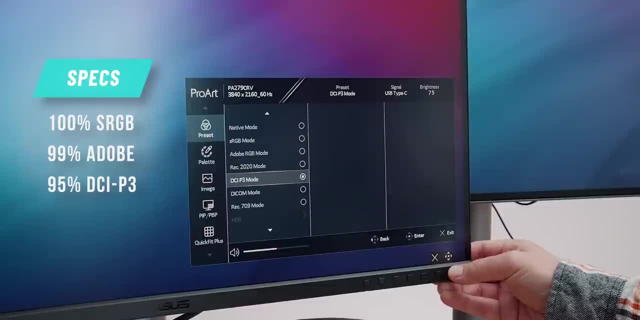 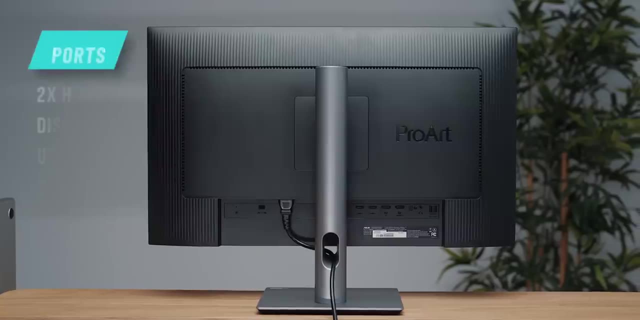 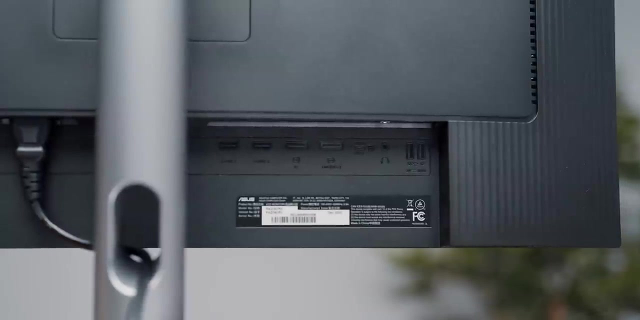 sRGB, 99% Adobe and 95% DCI-P3, it is, in fact, the leader of the bunch if we talk about numbers. only Keep that in mind. There are two things that make this monitor special, aside from the price, of course. First and foremost, it can output 96W of power, which is 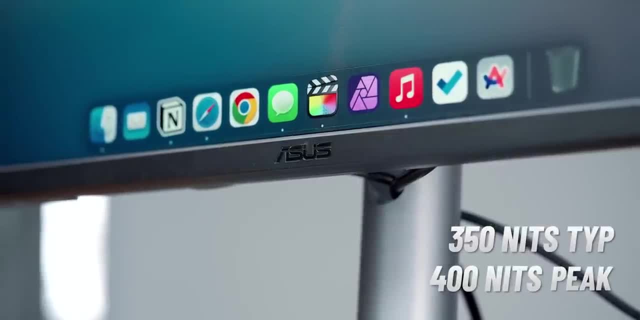 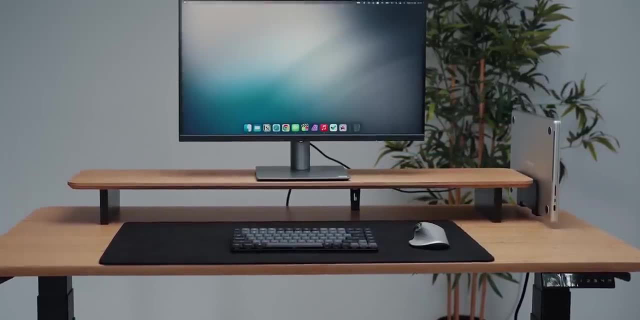 very surprising for this little guy. Second, it is a very bright monitor, providing 350 nits typical and 400 peak brightness. If you work in a bright office or studio, it does make a difference, believe me. Another thing I appreciate is the built-in power supply, Since the monitor is 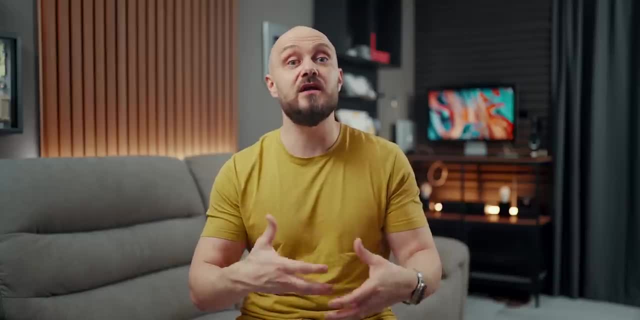 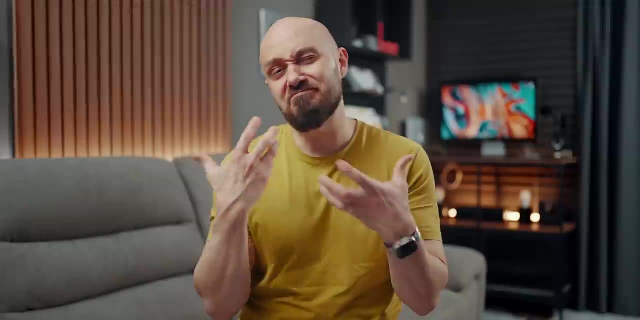 very light. you can easily mount it on an arm without worrying about any additional power bricks that you might have to hide somewhere. Now the lightness brings me to the shortcomings. This monitor feels very plasticky and the least premium of all four. 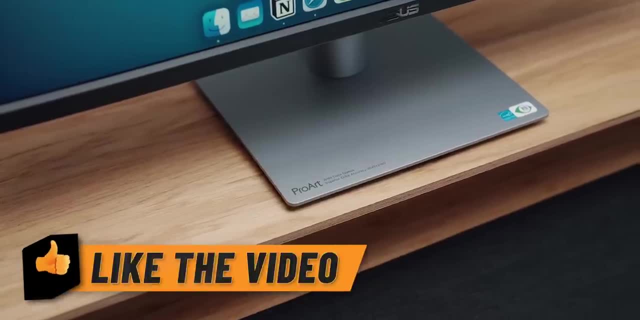 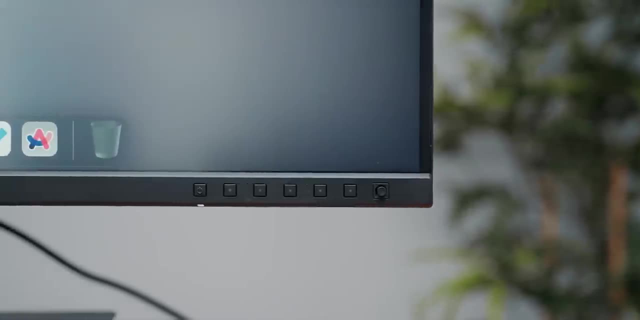 Not that this is a problem, but it's worth considering. The stand feels very 2013,, not 2023, and I don't like the chin, although I appreciate the easy on-screen button access. The biggest downside of this display, however, and it's totally justifiable. 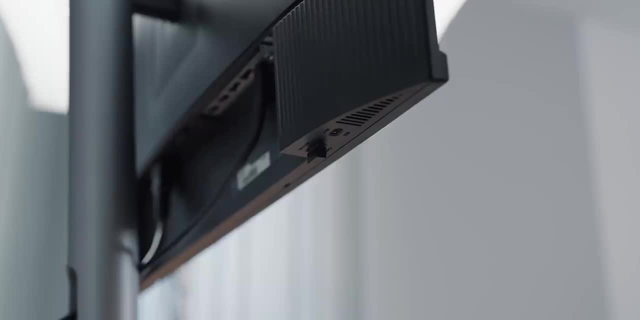 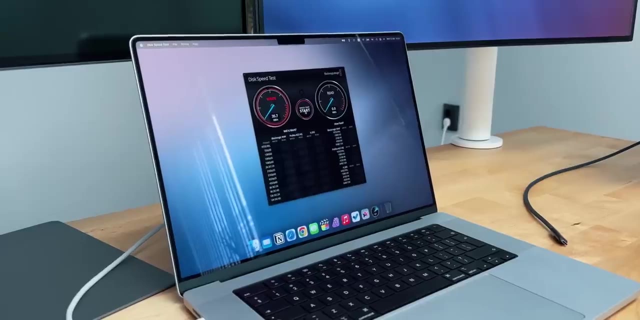 is the fact that it's not thunderbolt. That means that all additional ports will do a great job. if we talk about probably peripheral dongles and speakers, maybe You won't be able to plug in a drive and do much with it. Last but not least, there are no speakers. 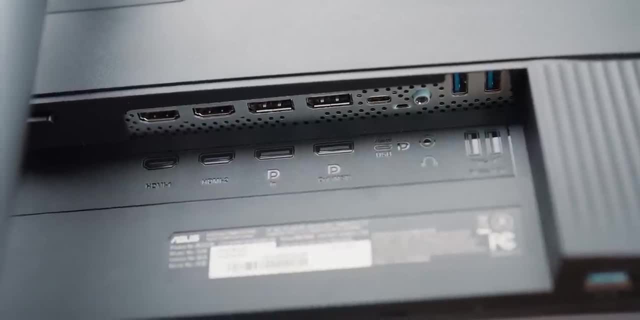 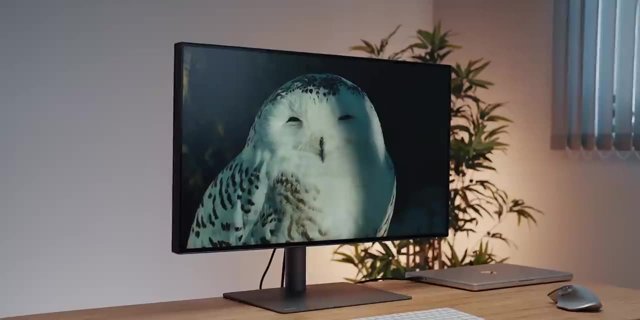 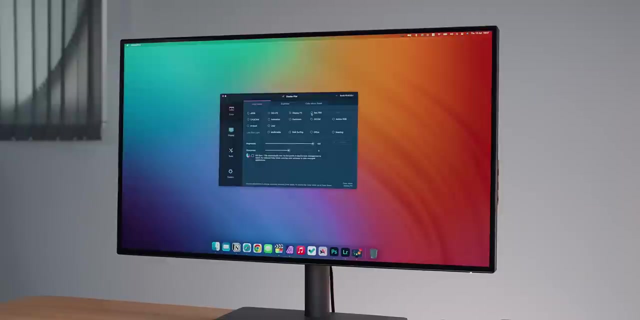 which I actually prefer, and I'll tell you why in a moment. Moving on to the versatility king, the BenQ. Equally impressive in terms of panel specs and, specifically, color accuracy, the BenQ shines with additional enhancements like the software tool called DisplayPilot. Aside from fidgeting with all sorts of picture settings you can assign. 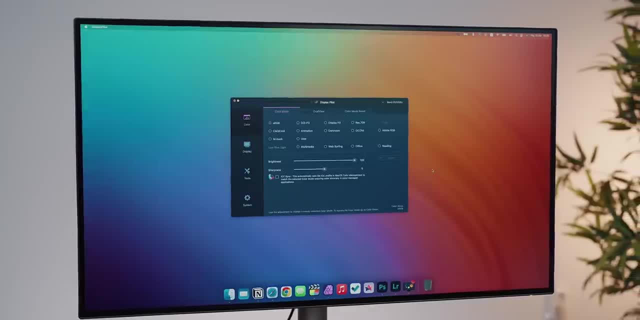 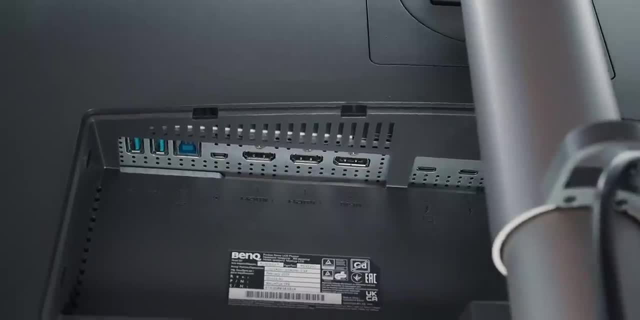 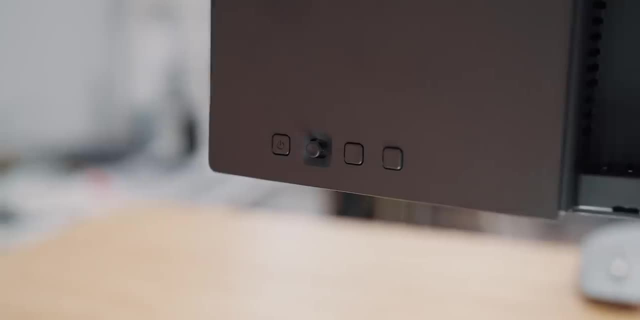 plugged in. for example, The monitor offers 85W power delivery to the connected laptop and it also has a built-in KVM switch allowing the user to control two systems like a Mac and a PC from one keyboard and mouse set, something you usually buy separately. 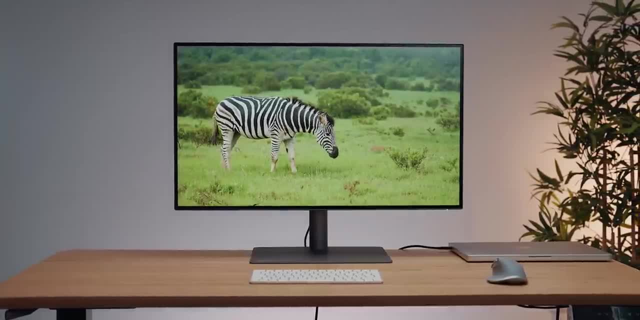 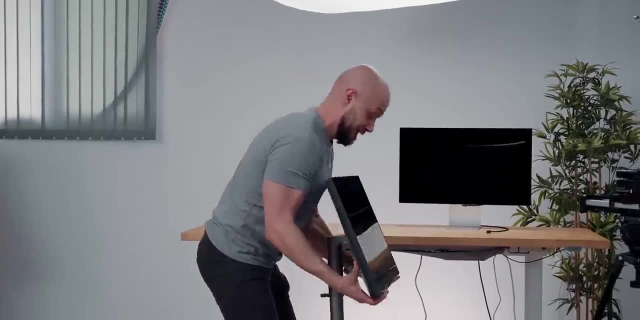 and it's awesome. Just as impressive is the size of this thing, which, honestly, is not something to brag about. It is so heavy that you have to go for a heavy-duty stand if you decide to prop it on a monitor arm. Also being so massive, one might think that it sounds. 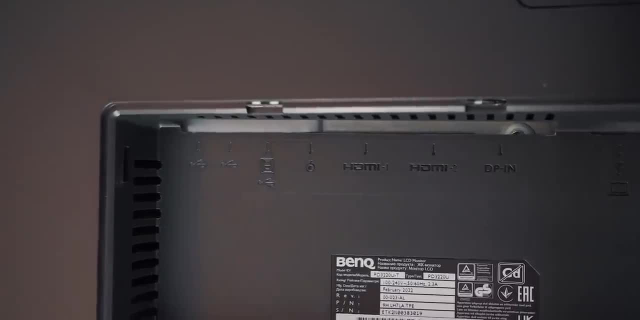 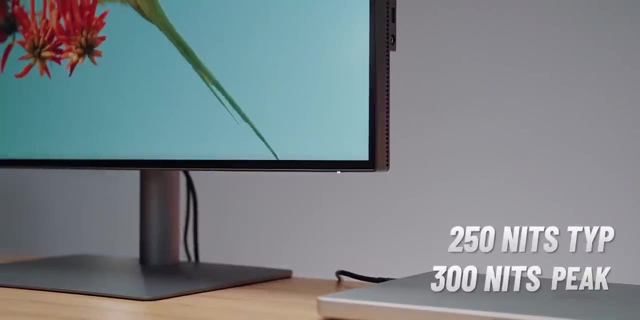 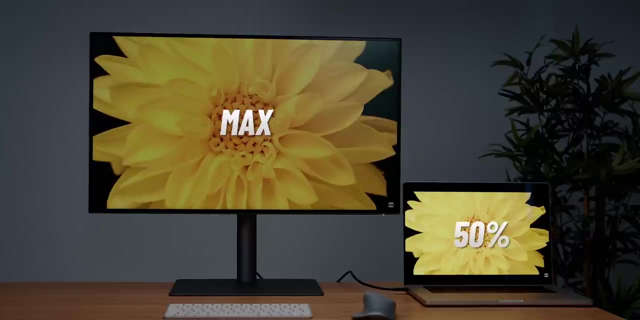 decent given all the internal dimensions, but in fact it sounds comically unimpressive. Finally, my biggest disappointment is the brightness At 250 nits typical brightness. my habits had me constantly smashing the brightness up button on the keyboard with the hopes that something would change If we have the blinds open. 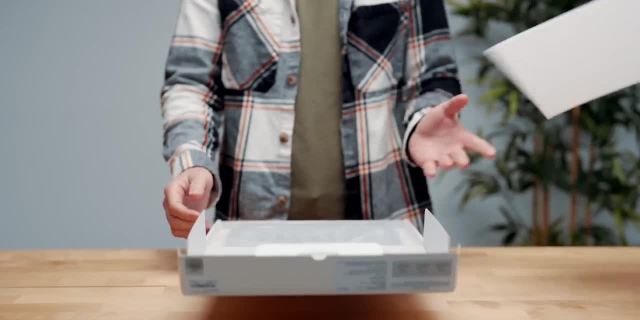 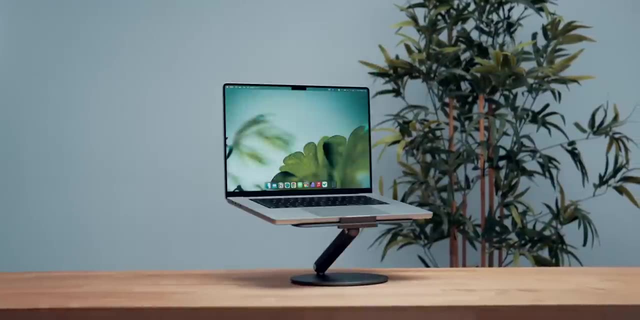 I would honestly struggle a bit. Before we move on, let me show you the Infinity Max laptop stand by Banks. It's a stand with a twist. At a glance it's a height and tilt adjustable stand able to accommodate pretty much any portable computer under 16 inches. When necessary, it can completely 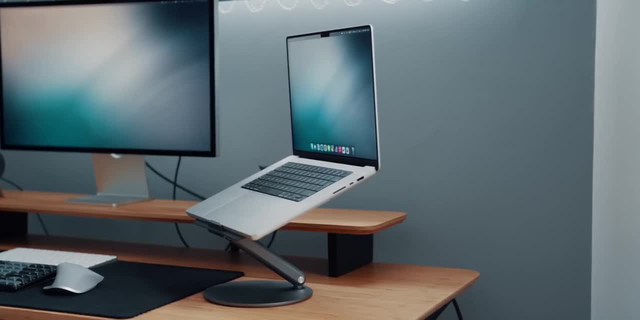 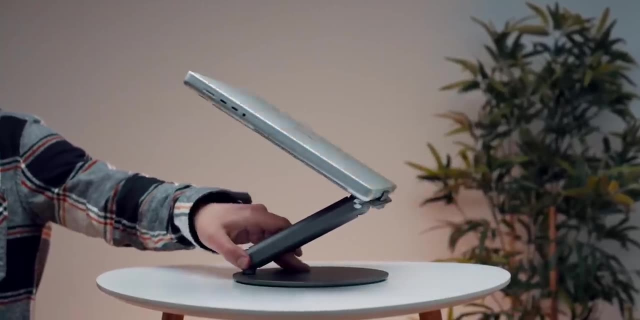 collapse for storage or on-the-go purposes, Designed to fit any work style and desk setup. aside from looking extremely elegant, it impresses with the cleverly designed 360 degree rotating base. It's super responsive and smooth, giving the vibes of playing with the most. 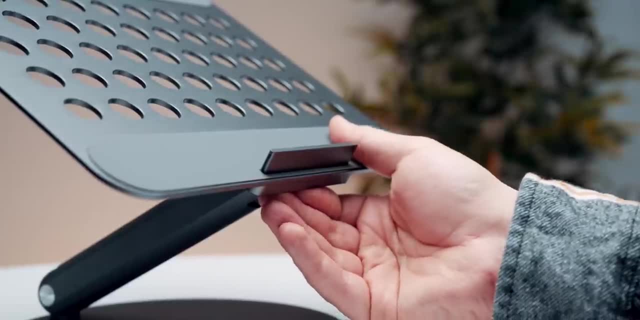 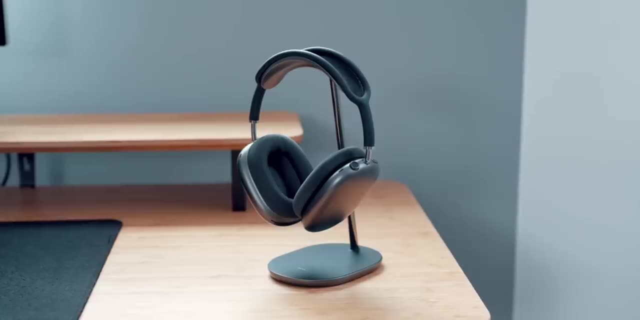 giant fidget toy ever. The adjustable front widget secures the device no matter the angle, while the main plate ensures great heat dissipation. To add even more style and texture to your workplace, you can bundle it up with Banks Grand Headphone stand, which is made 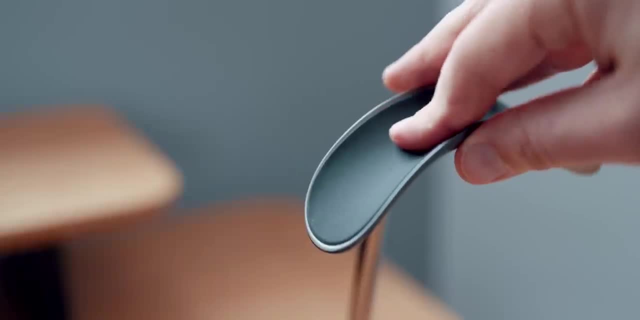 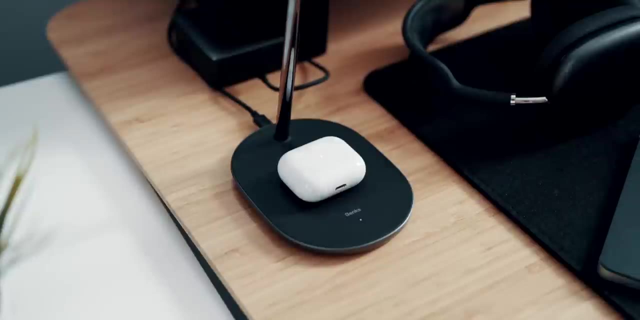 with the AirPods Max in mind. It's sturdy, yet super gentle, thanks to the silicone surface, which protects your headphones from scratches. As an extra perk, that stand can wirelessly charge your devices with 15 watts fast charging, which I definitely appreciate. 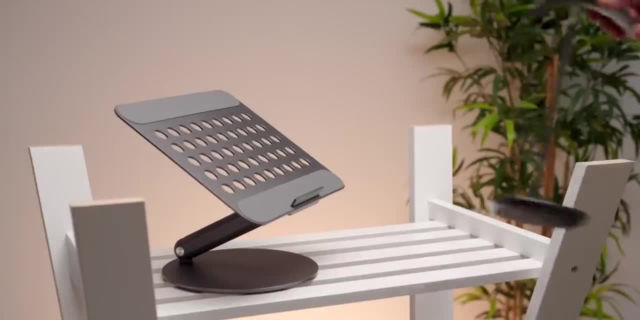 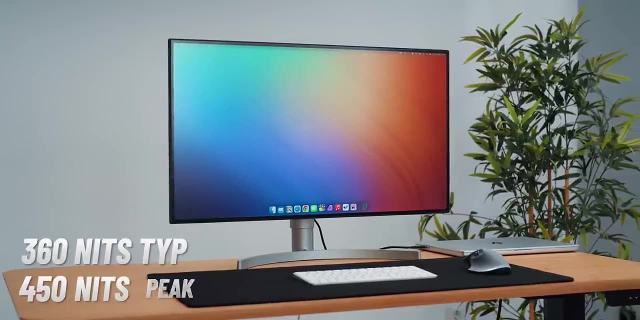 Be sure to check out the first thing in the description below to take advantage of Banks special offer on both stands. Next up is my old friend, the LG. I've covered this display extensively and still use it because it's great. It's a 5-year-old display at this point, yet LG still. 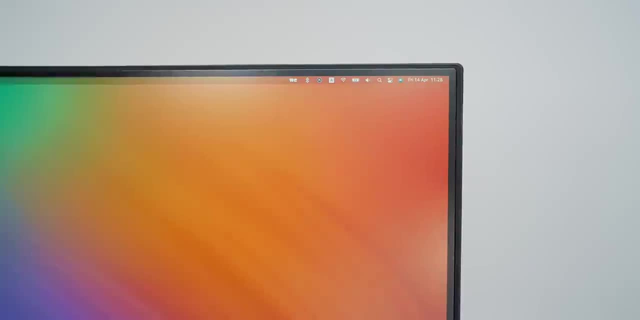 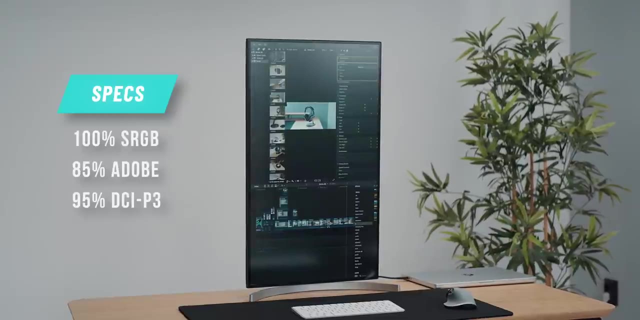 keeps it on their roster because it has everything you might require, including elegant and even front bezels. You can prop this display both horizontally and vertically and it will look amazing. It's the second brightest display after the studio display, yet it offers the slowest charging capability at 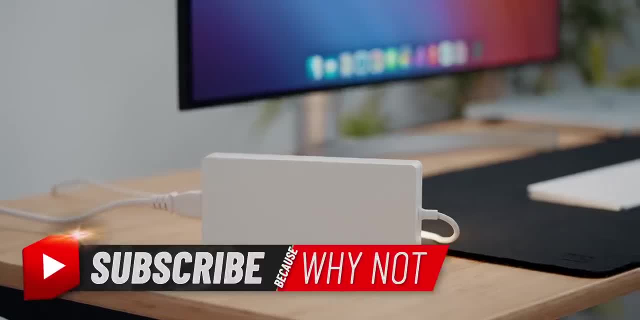 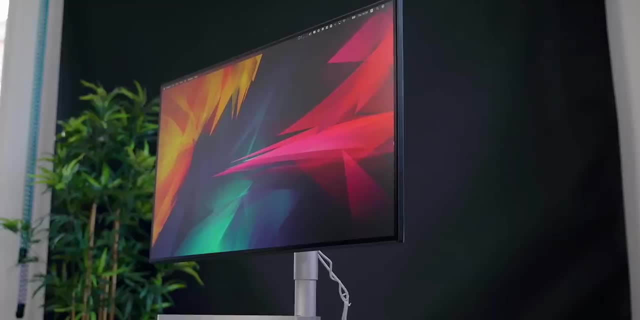 60 watts. What I don't like about it is the external power brick, actually, and the OEM stand, which takes too much desk space, if you ask me. but, as always, monitor arms. Feel free to check out my full review in the description below, but don't laugh at my newbie. 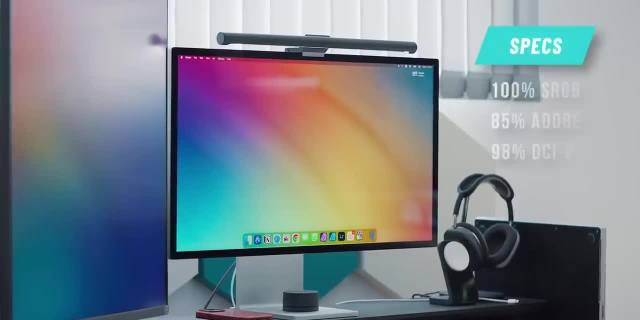 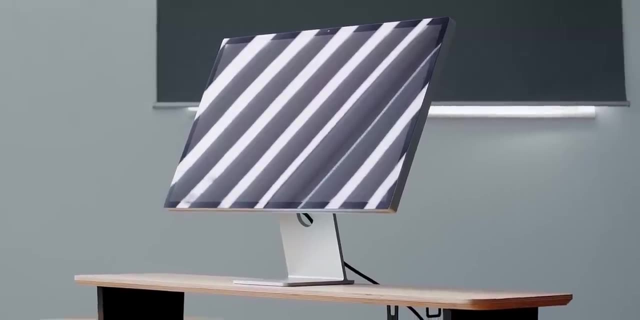 YouTube self from back then. The Apple Studio display impresses with unmatched build quality and aesthetics. Like its predecessor- actually this one, the studio display, will look good even after 10 years from now. yet you might still remember how much you paid for it. 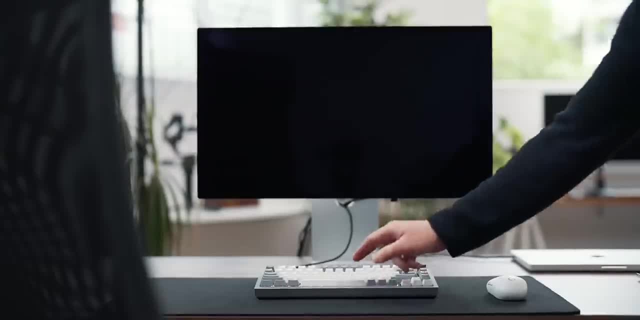 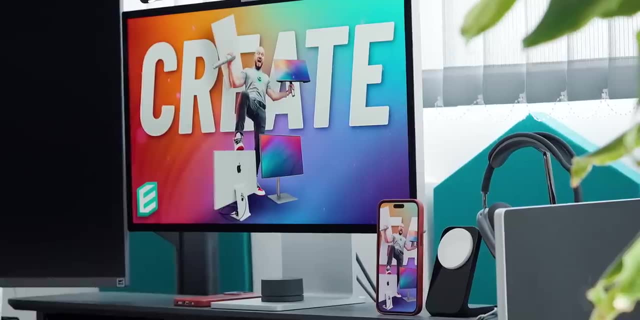 This is the fastest booting up display of them all, by the way, but even more impressive is the stunning picture quality. If you have any of the latest iPhone 13 or 14s, this is the one you can expect in terms of picture. yet in 27 inches It is plenty bright, at 600 nits, and it 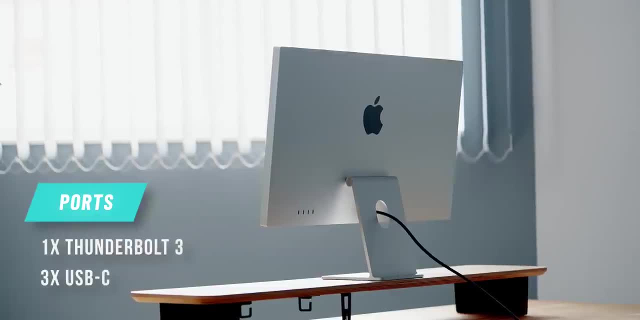 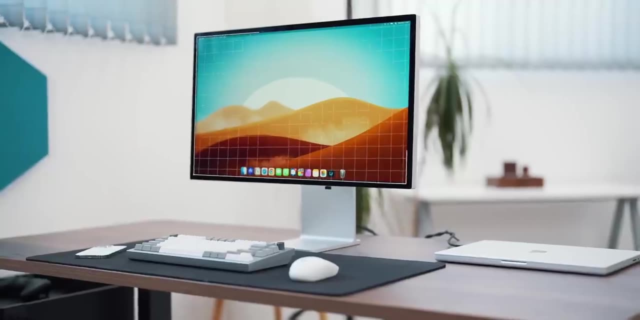 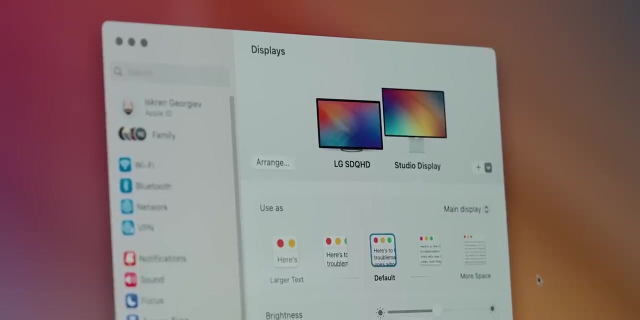 provides 96 watts of power for the laptop. The built-in speakers are unmatched in the category of monitor speakers, as is the 5K picture. Mac OS is designed to work in 1440p scaled environment, also known as 5K native resolution, so in 5K you can expect plenty. 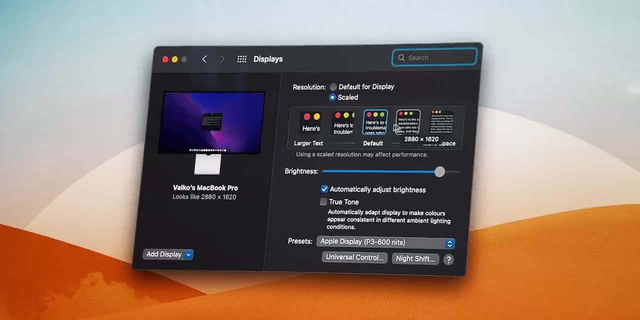 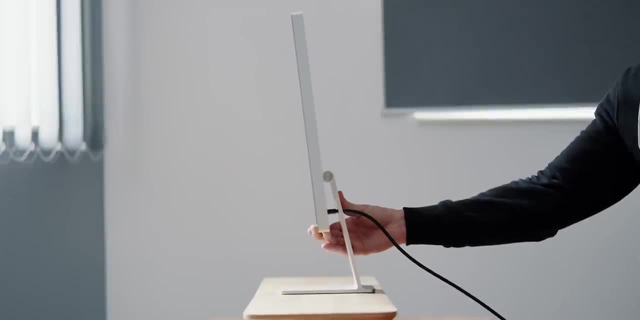 of real estate. crazy sharp PPI and no GPU pressure by default. Not everything of the course is sunshine and rainbows. though. You can't mount it on an arm unless you pre-order it that way. The ergonomic stand will cost you an Apple premium and the monitor is the least versatile. 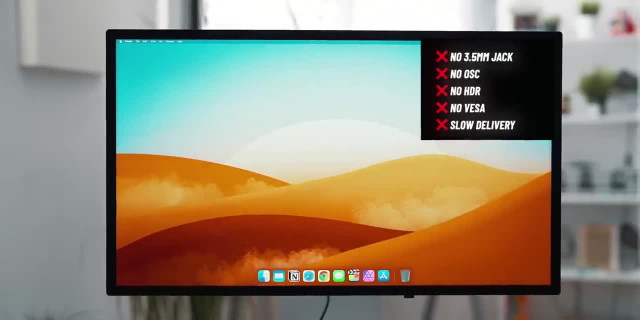 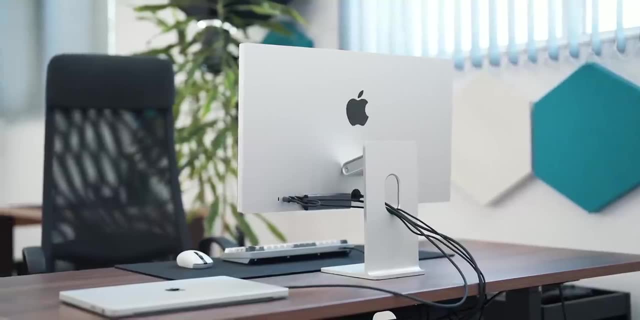 of all, Think of it this way: you have a Mac, you have a studio display. That's it. You can't have a studio display and have a PC or a Switch or any other console for that matter. You can just use this monitor with a Mac and maybe an iPad, but no multiple inputs. 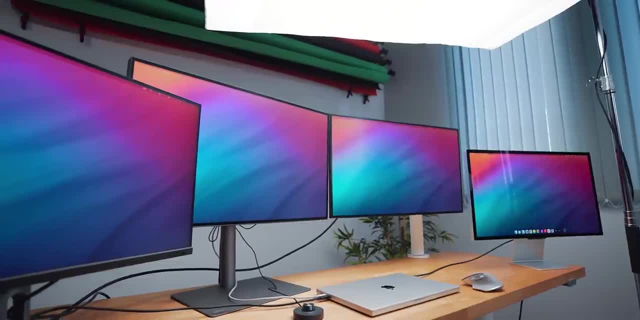 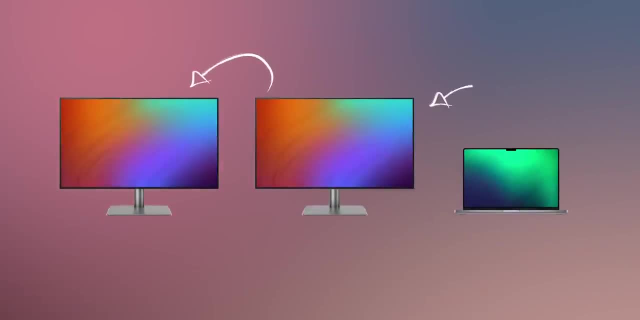 In terms of extra features, all four monitors have something to impress with. For starters, all the monitors, with the exception of the studio display, offer daisy chaining, the ability to connect a display to the main one and plug in just a single cable to the computer. However, all three 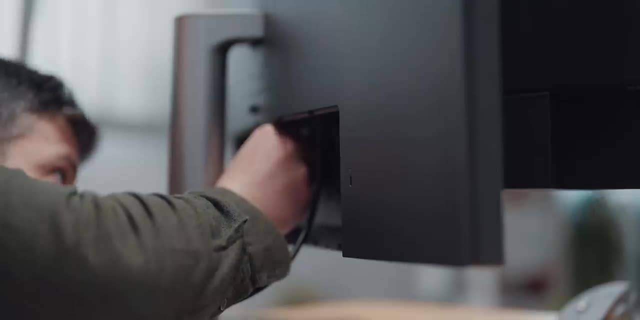 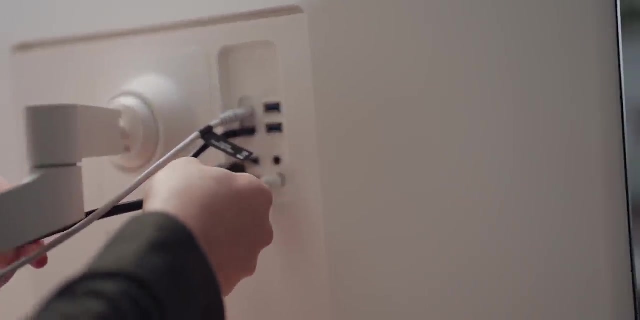 are very picky when it comes to that feature. Perhaps they work flawlessly if we daisy chain two of the same monitor models. but daisy chaining random brands, like I did in my tests, really depends on proper cables, multiple restarts and a little prayer. The Asus 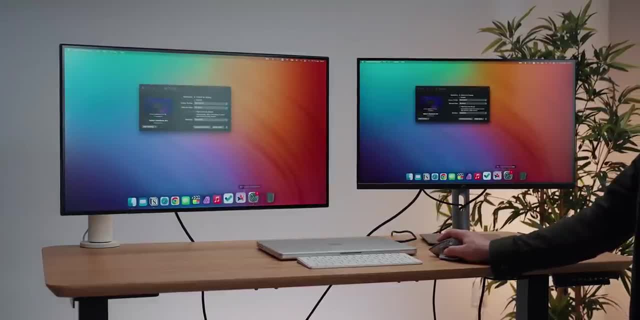 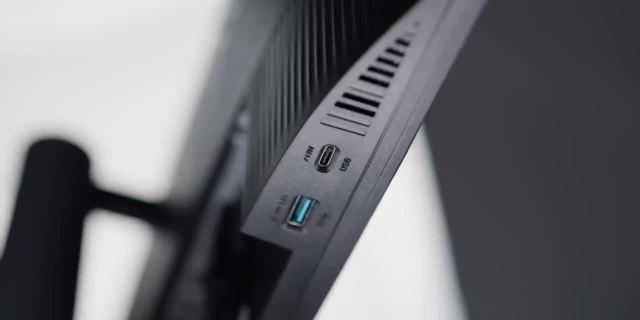 for example, was only able to mirror itself without being able to extend the secondary display. But this $500 monitor shines with the plethora of ports, including additional ports on the bottom left, where you have a USB-A plus USB-C, which offers 15 watts of power. 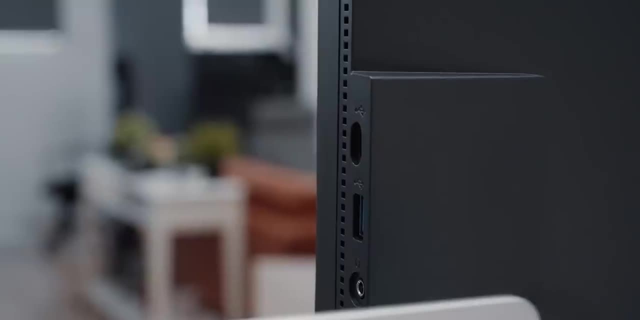 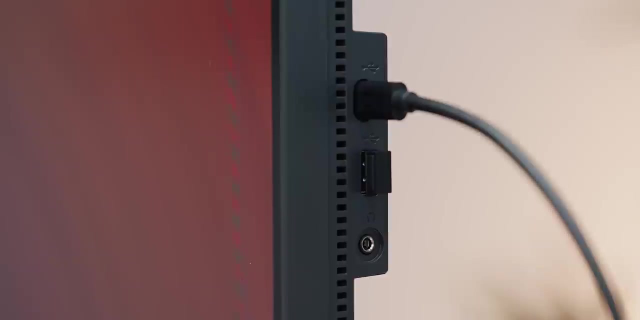 great for plugging in and charging your phone, for example. The same extra ports are available on the BenQ monitor, yet on the side where one can find the headphone jack. Now, to be honest, this is not the best place for a headphone jack to exist, since, even if you decide to plug in your headphones, it would still be too far. If we talk about the price, it's a little bit more expensive than the $500 monitor, but it's still worth the money. You don't have to worry about the price, but it's still worth the money. You don't have to worry about the price, but it's still worth the money. 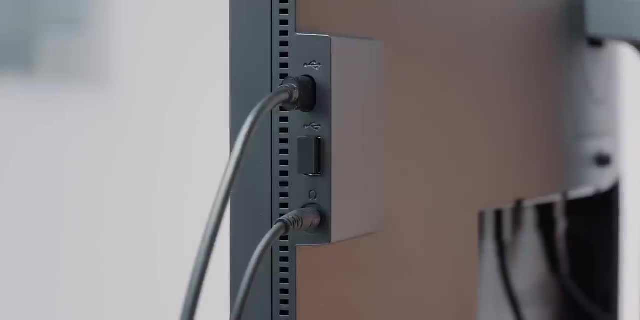 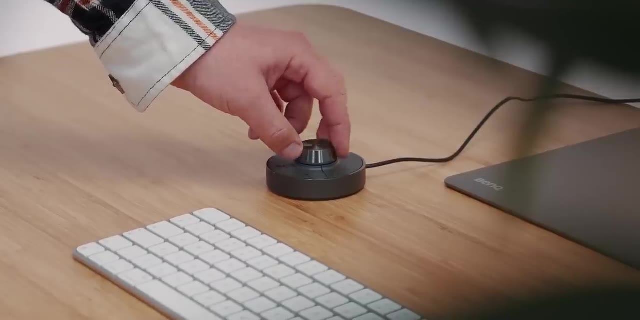 If you decide to plug in your headphones, it would still be too far. If we talk about external speakers, you cannot possibly achieve a clean setup with those cables coming from the side. The side ports should be more of a temporary port, if you ask me. Needless to say, BenQ also. 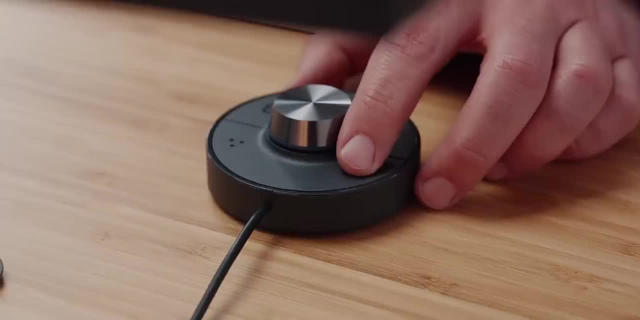 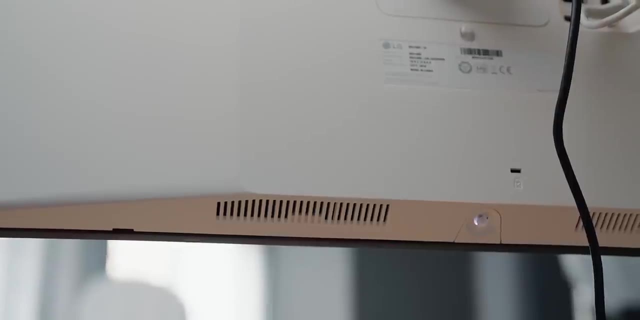 shines, with the additional hotkey puck which sits neatly towards the user, allowing instant adjustments. The LG monitor doesn't have any groundbreaking perks to brag about, aside from being the Gandalf in this group, but out of all, it is the most elegant-looking. 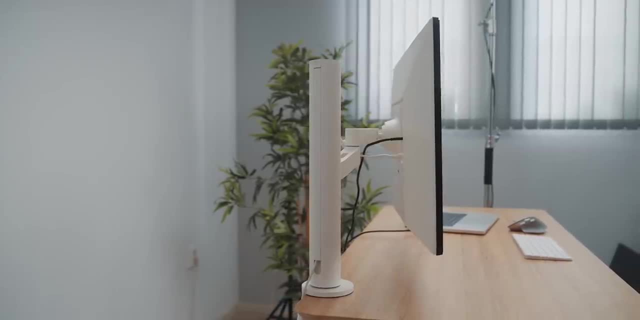 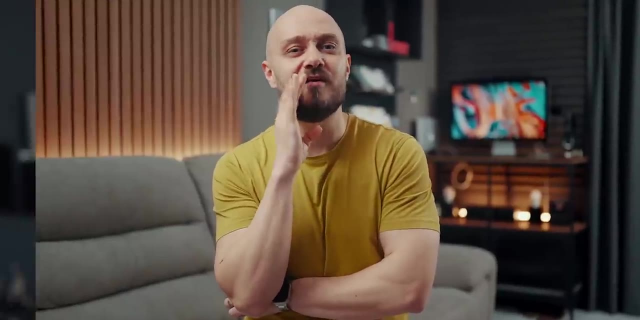 with its thin profile and even bezels, especially on this ergo arm. The arm, by the way, is not part of this particular model, but just between us. I can't remember where I've placed the original stand, which I don't use because it takes too much desk space. 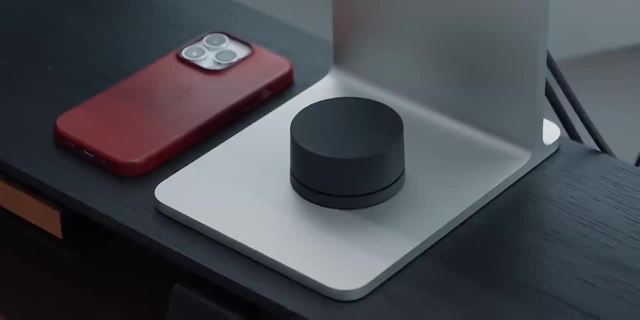 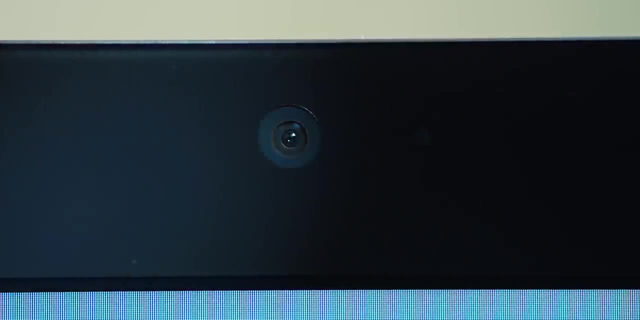 Ok. so the Apple Studio display can flex. with the 1080p built-in FaceTime camera and amazing microphone array With the A13 chip, the monitor is capable of delivering a decent picture for meetings with very good sound quality, But where it really shines is the speakers. 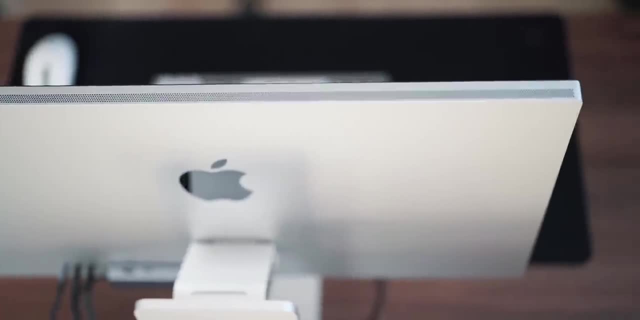 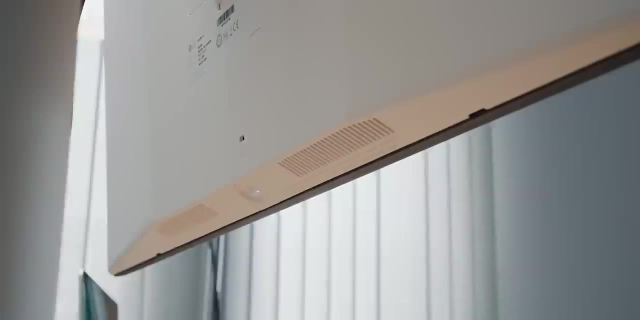 I have two pairs of studio monitors which I keep in my storage because the speakers on the monitor are amazing, Which leads me to speakers Aside from the studio display. the LG monitor is the second in place when it comes to sound, yet it's far behind what Apple have created. 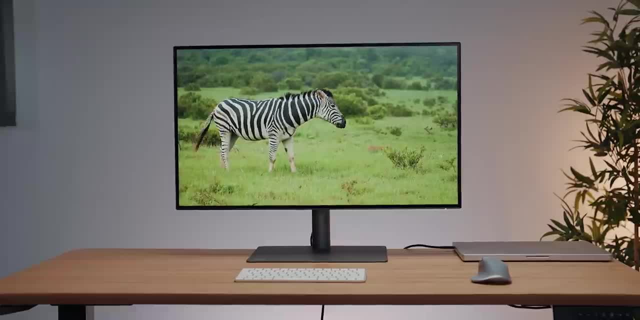 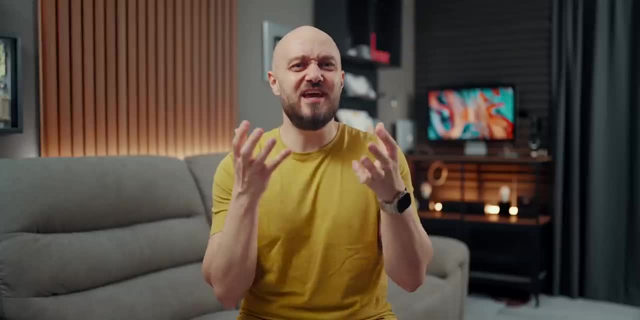 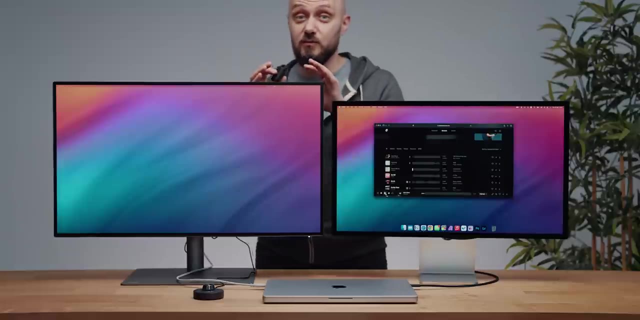 It sounds like a monitor, nothing more. BenQ, on the other hand, sounds like a $5 radio, Tiny teensy sound that I honestly didn't expect from a display that has such a thick and sheer presence. Ok, so I'm going to compare the speakers of the Apple Studio display and the BenQ monitor. 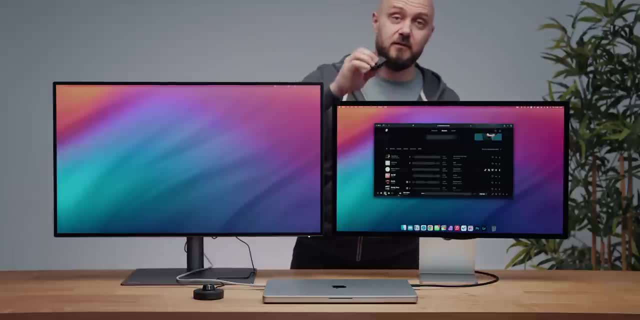 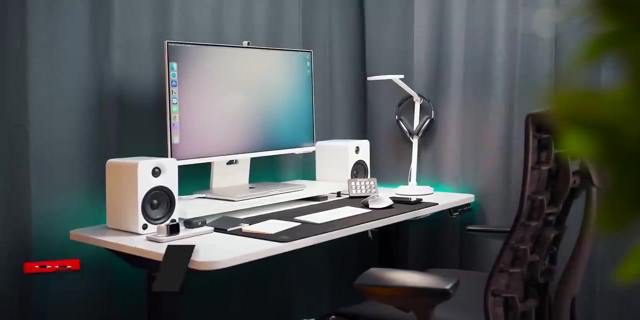 Let's start with the Apple Studio display first. Ok, so now let's switch to the BenQ and see the difference. The Asus has no speakers at all, and you know what? I'm totally fine with that. Like I mentioned in my Samsung M8 review, which I'll link below, I prefer no speakers and a headphone jack than